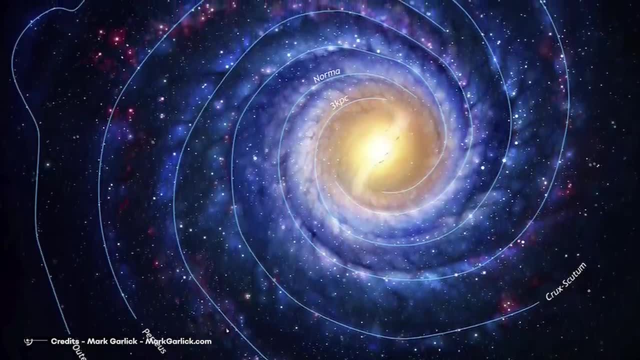 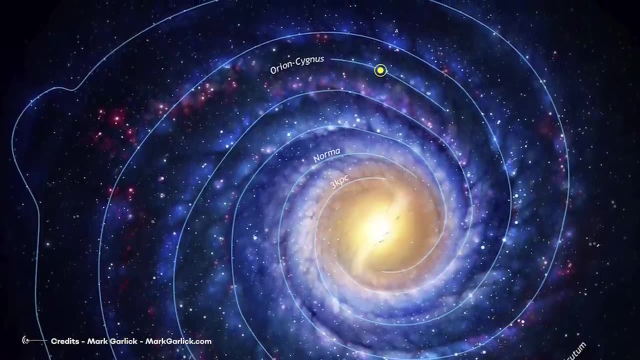 A new discovery suggests that one of our galaxy's spiral arms, located some 4,000 light years from Earth, is jutting out at a weird angle. They're calling it a break in one of the Milky Way's spiral arms. Keep watching the video to get to know more about this unexpected break. 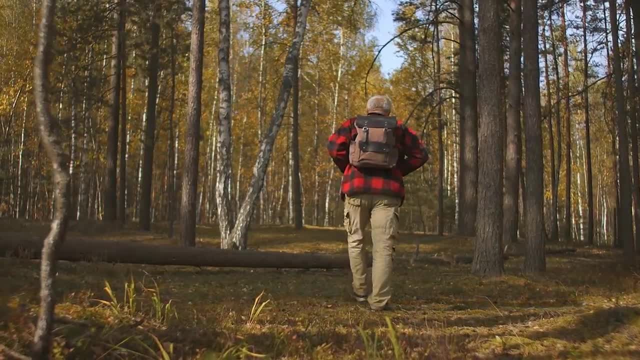 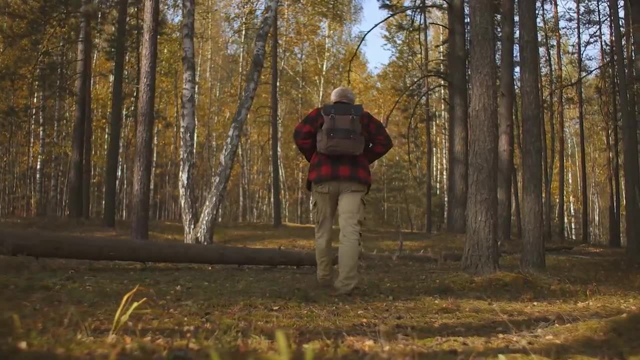 Imagine being alone in the middle of a forest. You're surrounded by all kinds of trees and you have to hurry up because the night is coming and it would be very dangerous for you to stay there when the sun will be gone. How could you tell where there's a way out? 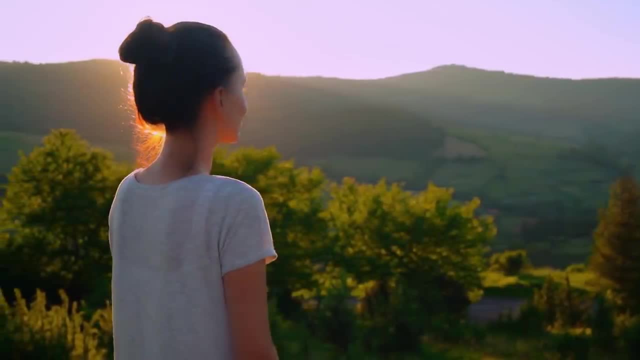 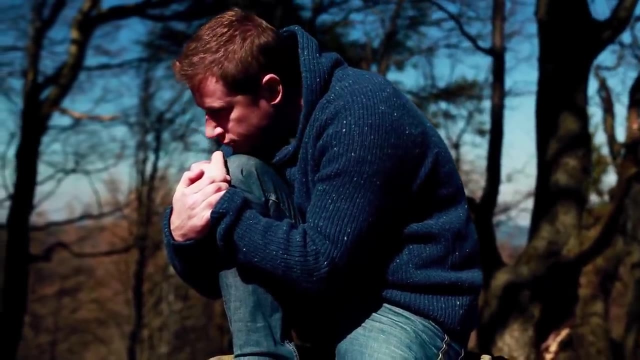 If there was a friend of yours watching you from a top view, he would have perfect control of the territory, so you can ask him to guide you out of there. But suppose you have no friends unless you are very lucky or unless you are Bear Grylls. 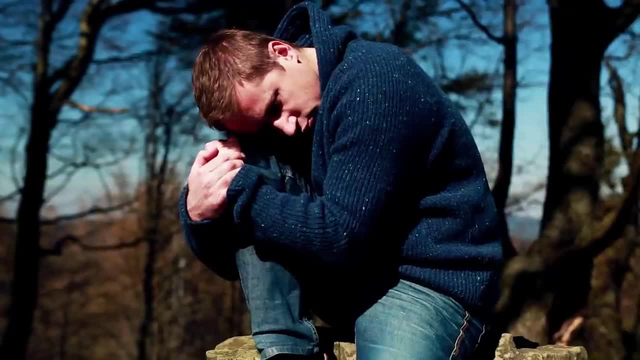 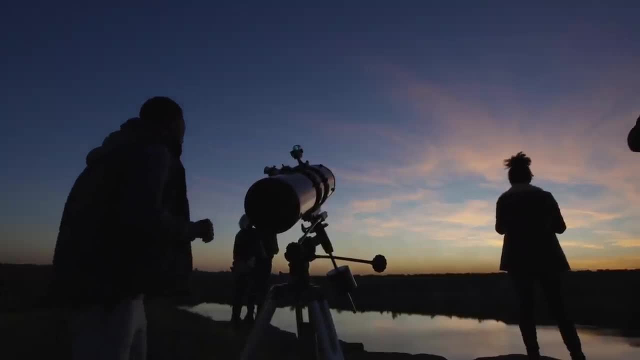 You're gonna probably be stuck there because you simply can't see the forest for the trees and you have no chance for a top view. Well, this is pretty much the same situation that astronomers face when it's time to understand how our galaxy is. 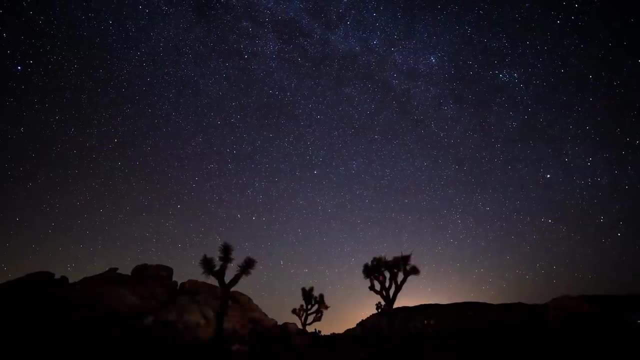 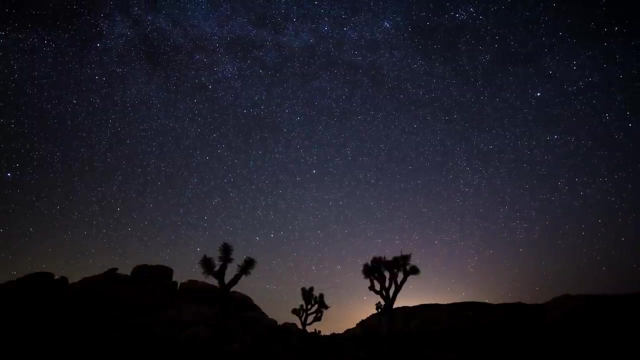 Sometimes you can't see the galaxy for the stars, Because we're inside the Milky Way and we can't get a complete view of the forest of stars surrounding us. This is why it's so difficult to understand its properties and features, And when a team of astronomers starts studying. 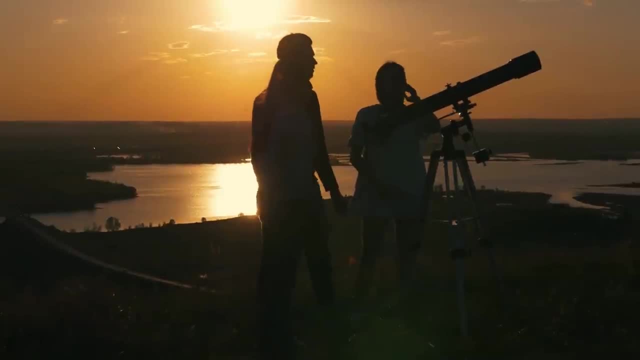 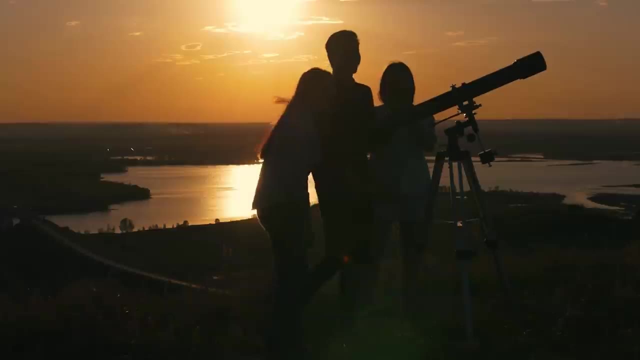 in detail some part of our galaxy. it means that it's probably time for new discoveries. Astronomers from all over the world weren't surprised to hear that we found a break in one of the Milky Way's spiral arms, But what is it? 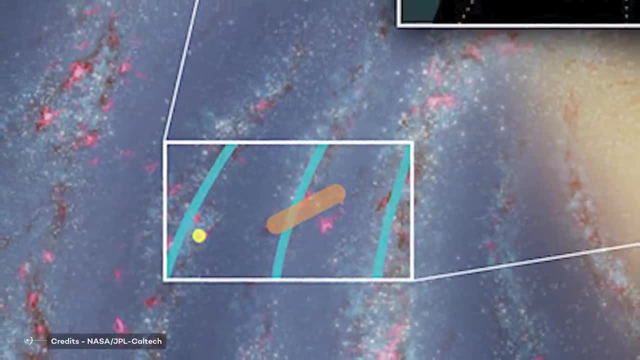 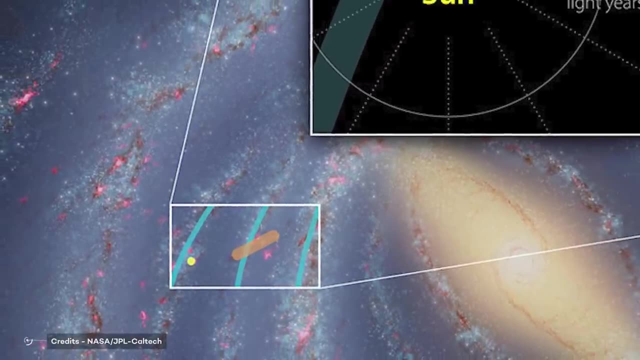 Well, this break, which extends from the Sagittarius arm of our Milky Way galaxy, has a strange orientation. Of course, other pieces of spiral arms exist with very peculiar orientations, but this is the first major structure identified with such a dramatic one. 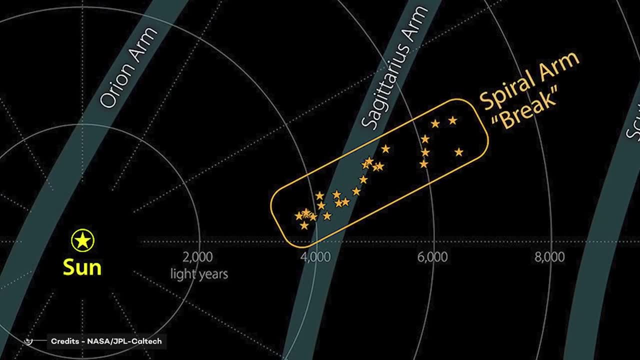 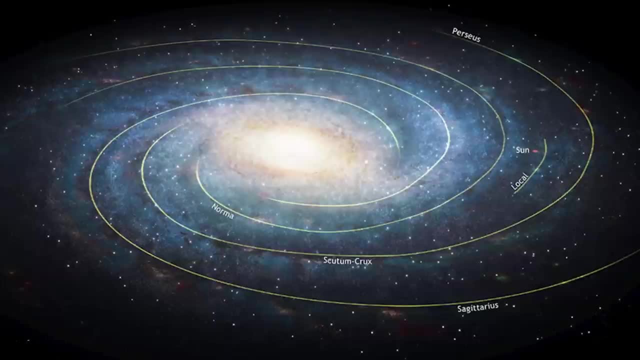 The scientists published their discovery on July 21, 2021, in the Pure journal Astronomy and Astrophysics. Let's try to understand where this break is located. We could say that the splintered region of the Sagittarius spiral arm extends for some. 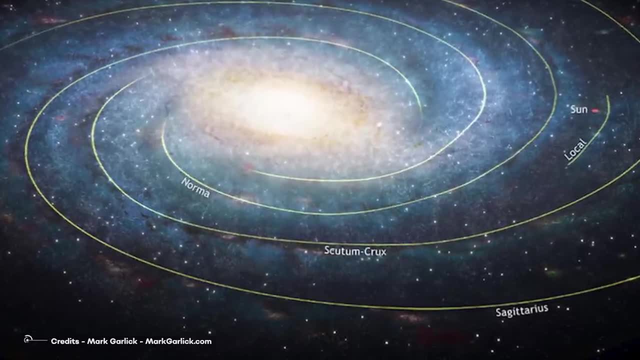 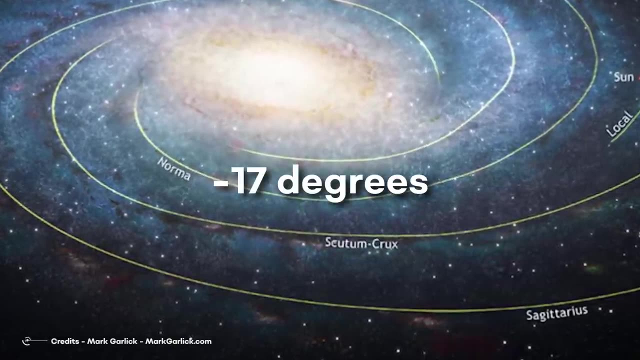 3,000 light years at a sharp angle from the main arm. that is the tangent to the start of the Sagittarius spiral arm, which lies at a galactic latitude of about minus 17 degrees. But we're not astronomers and these numbers are not telling us much. Maybe things are. 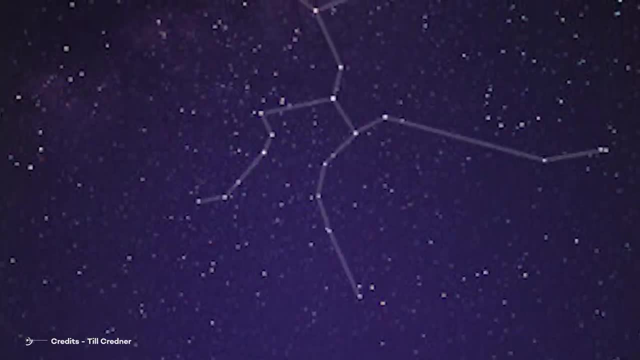 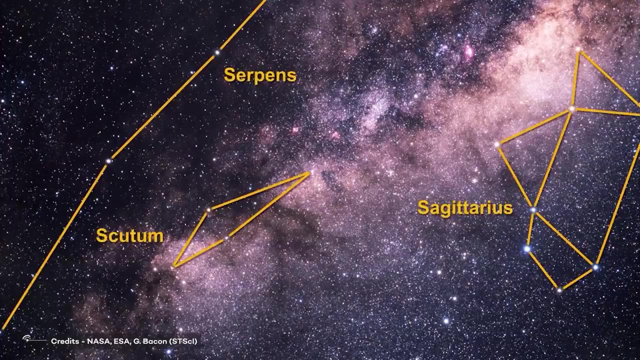 clearer if we talk in terms of constellations. That region of sky is the region we're looking toward when we gaze at the constellations Sagittarius and Serpent's cauda and the Milky Way that flows behind these stars- Some of the stars in nebulae located in the 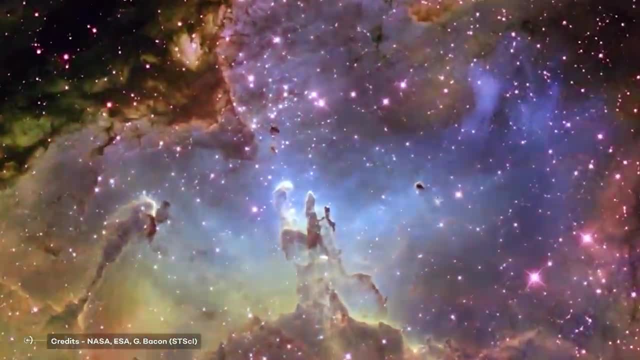 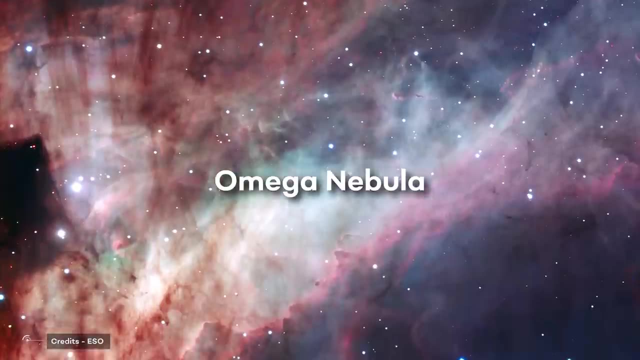 spiral arm break are the most famous in the heavens. They include the Eagle Nebula, which is known for the Hubble Space Telescope's Pillars of Creation photo, and it includes the Omega Nebula and the Trifid Nebula and Lagoon Nebula. 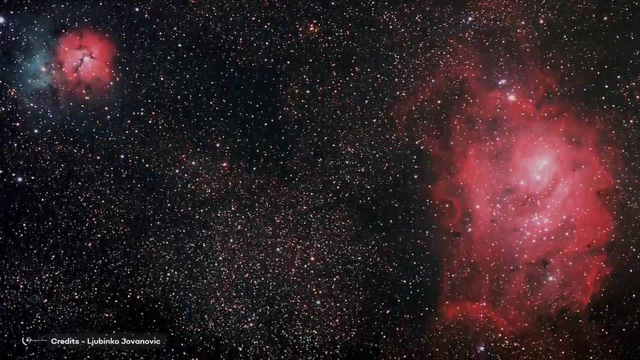 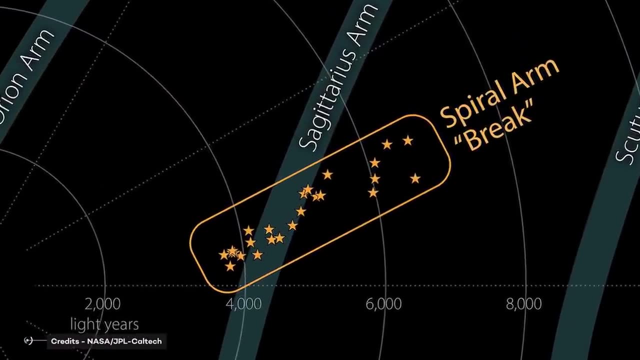 These nebulae are often photographed together. Here we are Now. you get me. Now that we know what the break is and where it's located, let's see how scientists found it. Of course they needed a telescope, or better to say, 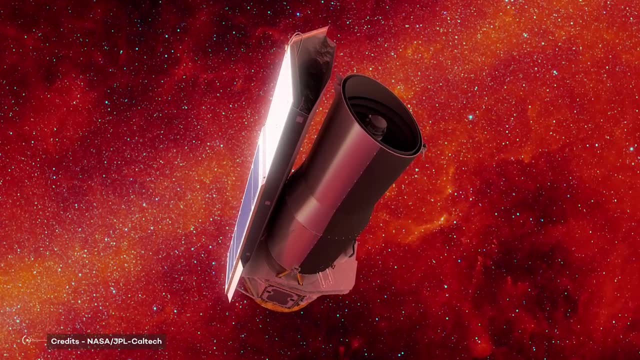 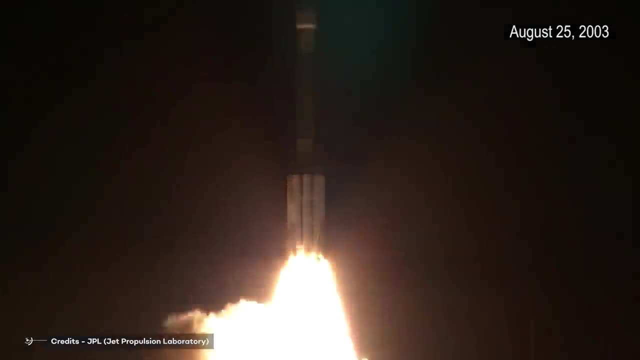 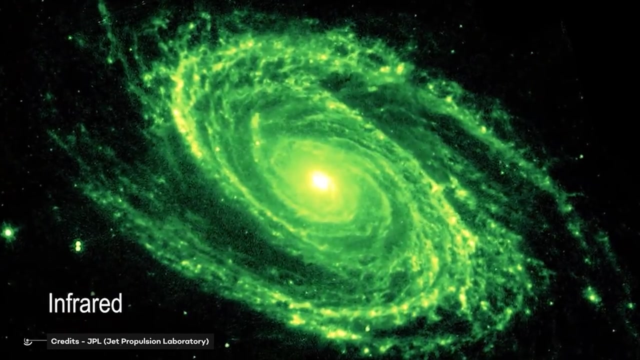 they needed data from a telescope. That's why they turned their attention to NASA's Spitzer Space Telescope, Launched in 2003,. NASA's Spitzer Space Telescope was the fourth and final addition to NASA's Great Observatory Program. NASA's mission was to become NASA's premier infrared light observatory, offering astronomers. 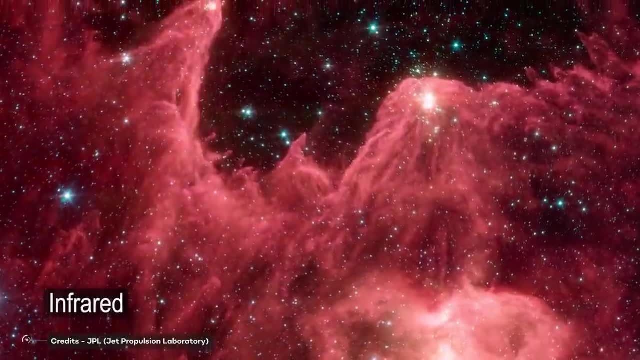 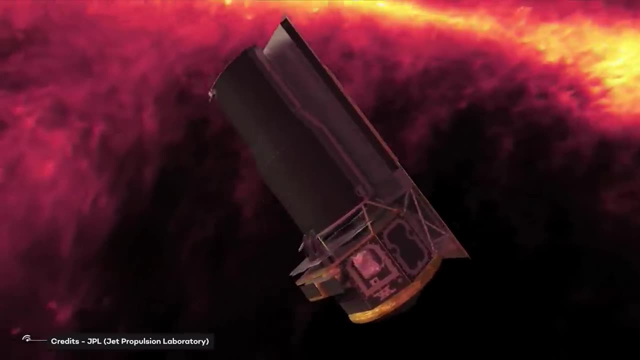 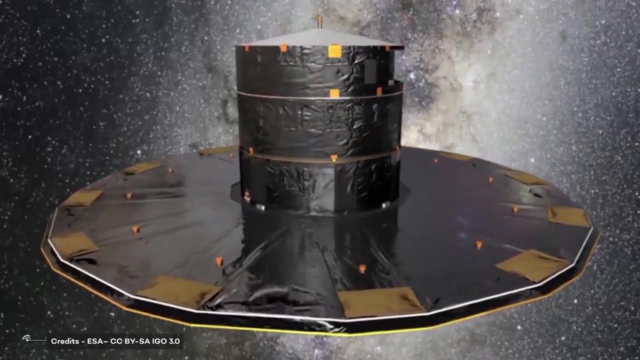 the chance to study the universe in this critical part of the electromagnetic spectrum of light with unprecedented clarity and sensitivity. Thanks to it, they analyzed a bunch of data regarding young stars that the telescope's infrared vision could see hiding within these nebulae. They also used data from ESA's Gaia mission to measure precise distances to the. 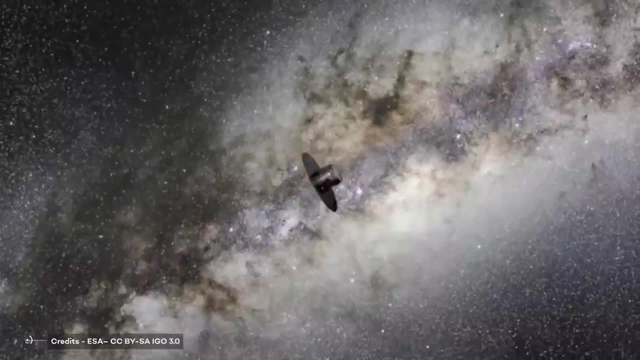 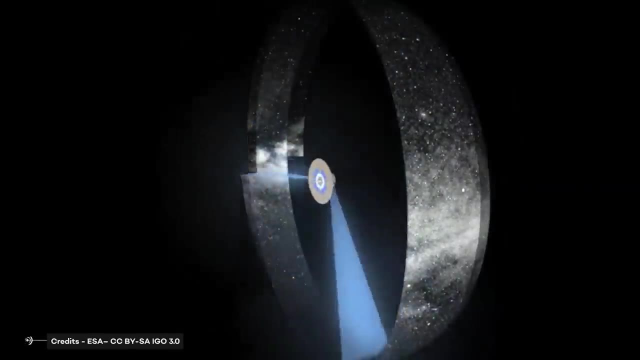 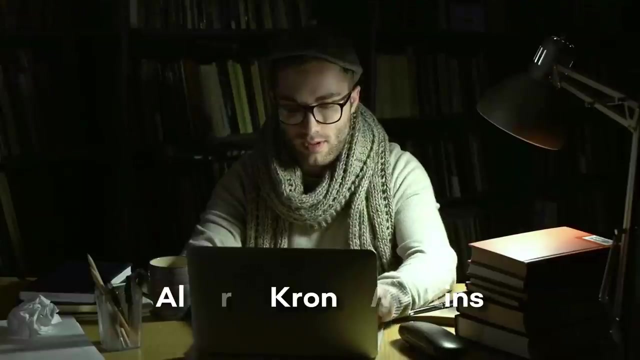 stars. Gaia is a very important instrument. It will lead astronomers from all over the world to a better understanding of the place we are living in and, more generally, our entire universe. It is so precise that some astronomers started using its data before they were made official. 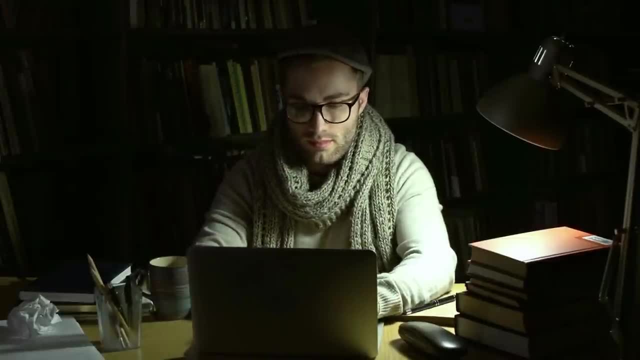 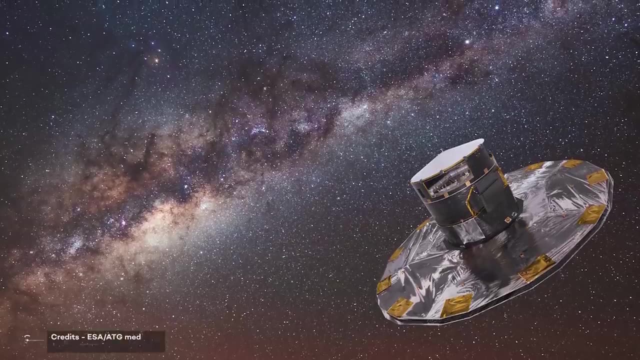 Alberto Cronos Martins, one of the authors of the study from the University of California, Irvine, said that distances are among the most difficult things to measure in astronomy. It is only the recent direct distance measurements from Gaia that make the geometry of the star. 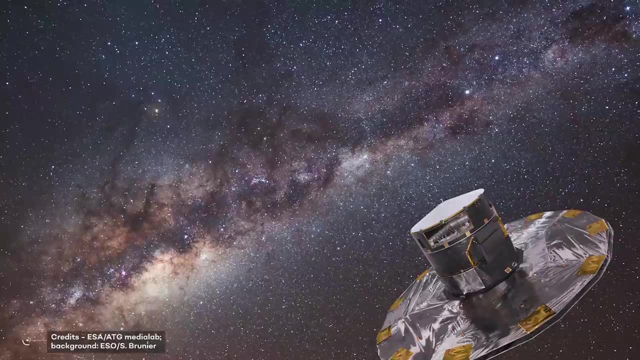 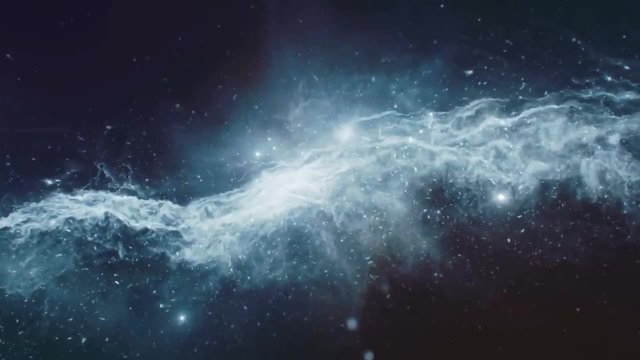 In fact, it is only the recent direct distance measurements from Gaia that make the geometry of this new structure so apparent. The combination of the two sets of data revealed that the splintered segment of the Sagittarius arm contains young stars moving at nearly the same velocity and in the same direction. 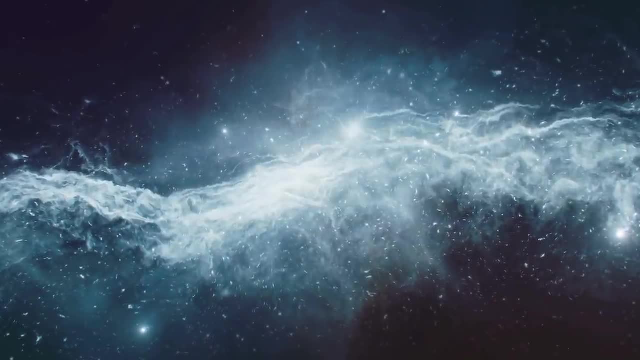 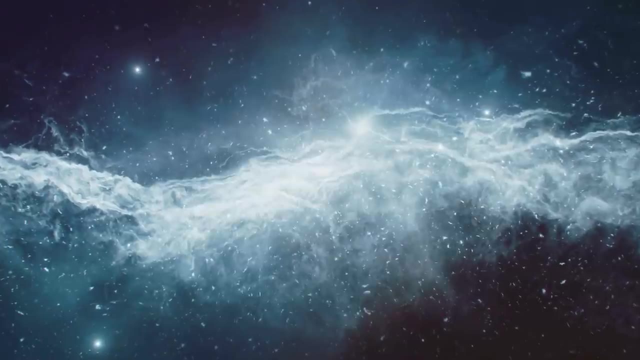 through space. When they put the Gaia and Spitzer data together and finally see this detailed three-dimensional map, they could see that there was quite a bit of complexity in this region that just hadn't been apparent before. The scientists do not yet fully understand why this is so important. The scientists are still trying to understand why the two-dimensional map is so important. The own star is a government for the production of the whopping star number of galaxies, And yet there is no way to understand the propensity of theбalance of all that material. 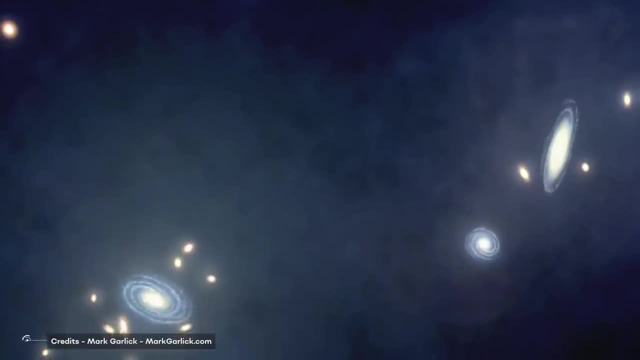 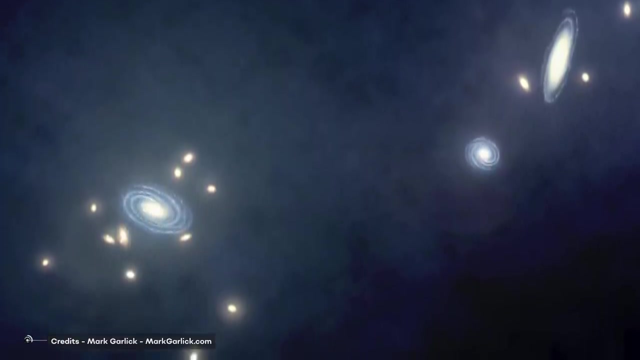 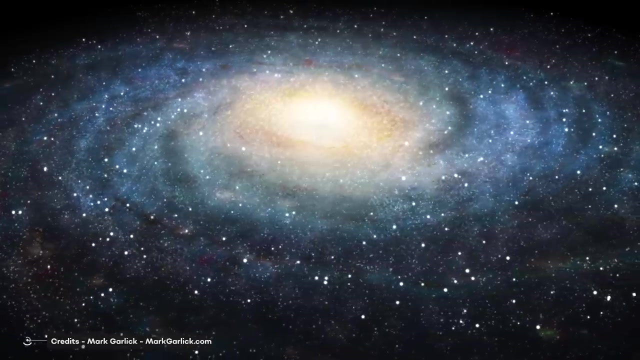 star material. While astronomers have discovered groups, local groups and clusters of galaxies in an estimated number of more than 100 billion, they have not been able to completely model and map out our own Milky Way galaxy, for the reasons we mentioned above. Ok, now that we know how this discovery was made, let's try to answer this question. 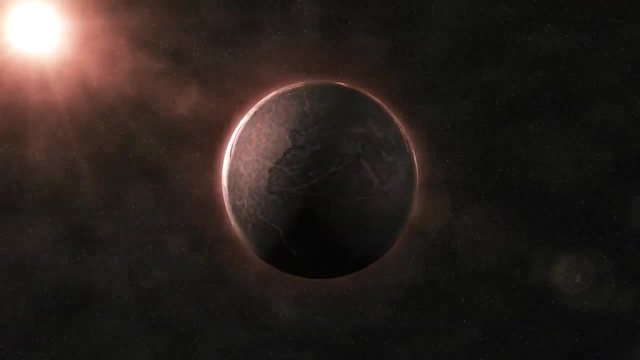 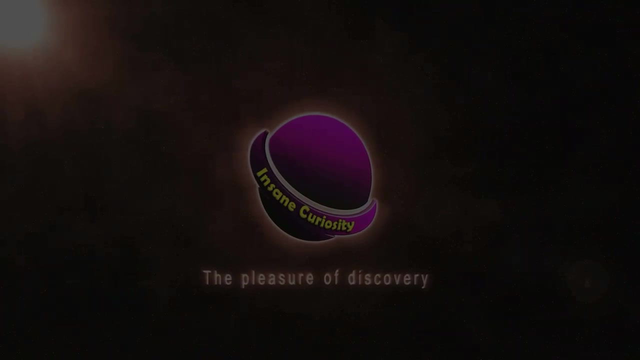 Why is the break important? Before finding out the answer to the question, be sure to like or dislike the video. video, so that we can continue to improve and make these videos better for you. the viewer Plus. be sure to subscribe to the channel by clicking the bell, so that you don't miss. 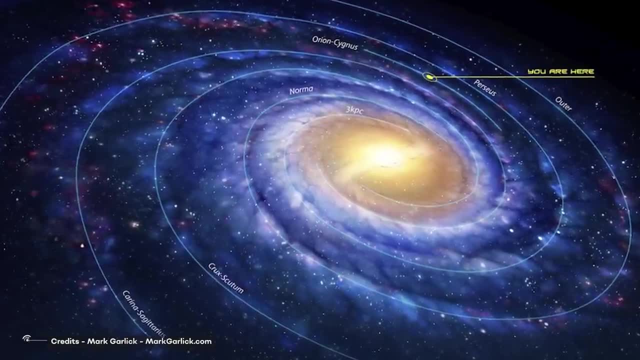 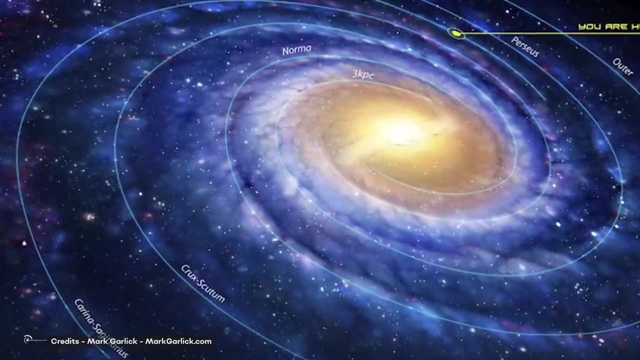 any of our weekly videos. Here's where you'll learn something new. today, The arms of a spiral galaxy are measured in something called a pitch. The pitch is set to be 0 degrees if the spiral is so tightly wound that it forms a circle. 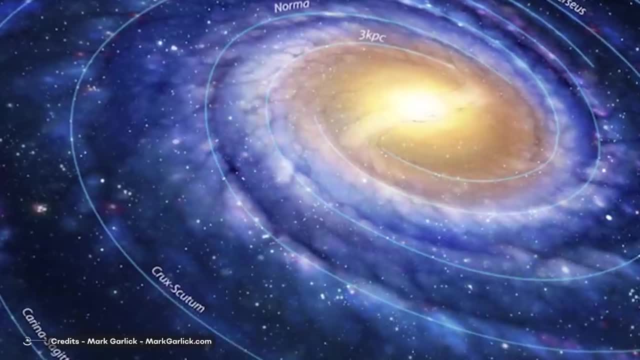 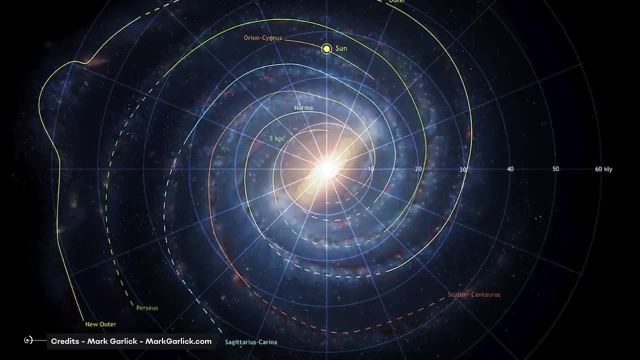 Instead, if a spiral arm opens up, the pitch goes up. Now, a key property of spiral arms is indeed how tightly they wind through a galaxy and what their pitch is. Analyzing the Milky Way's galaxy structure and putting all the physics we know in our 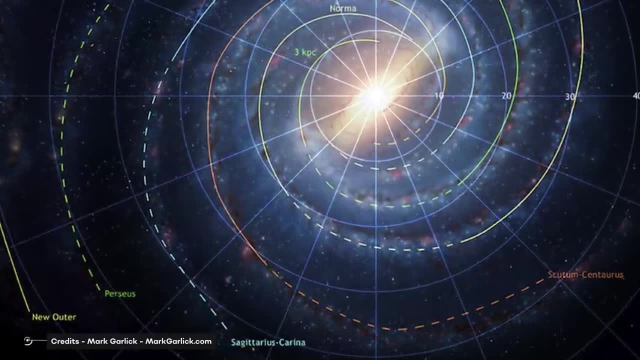 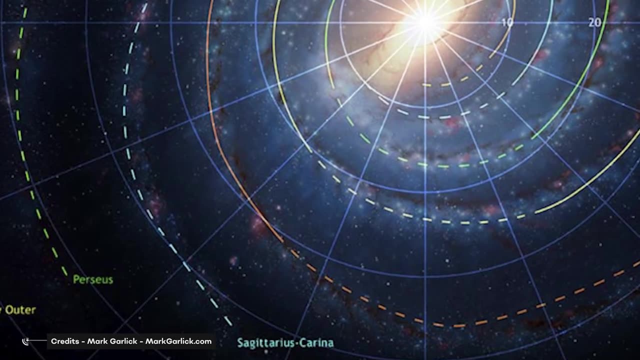 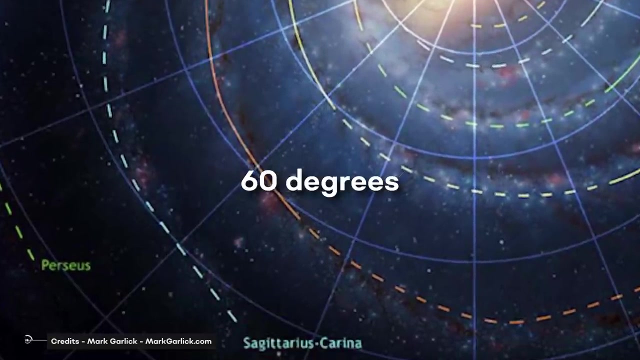 best stellar models. we found that the Sagittarius arm should form a spiral that has a pitch angle of about 12 degrees. But these were just models. The problem and the amazingness of this discovery came when they found the structure they examined really stands out at an angle of nearly 60 degrees. 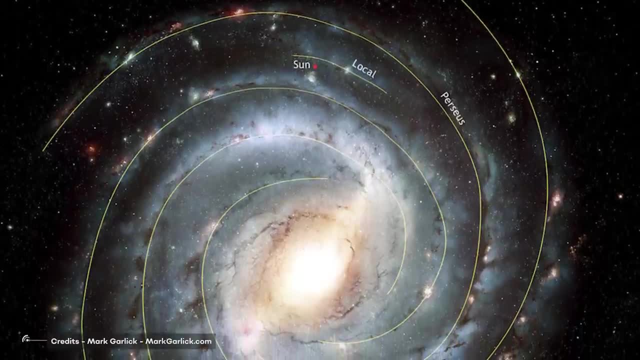 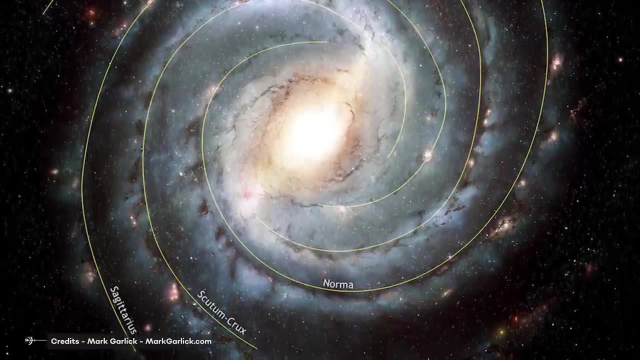 It's a huge discovery. It's a huge pitch. This spiral arm is very, very loose. Scientists have seen jutting breaks in spiral arms of other galaxies before, but this is the first time such a structure has been identified in our own galaxy.